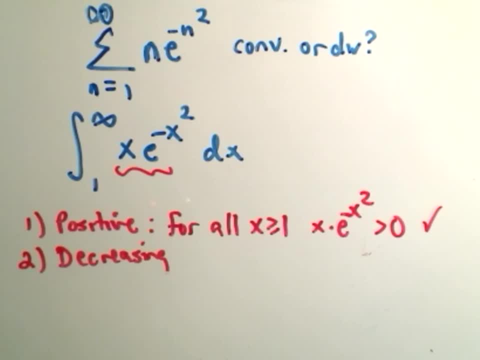 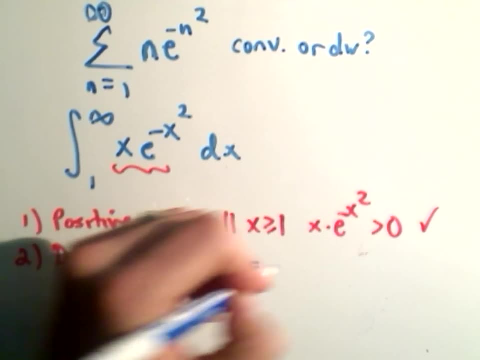 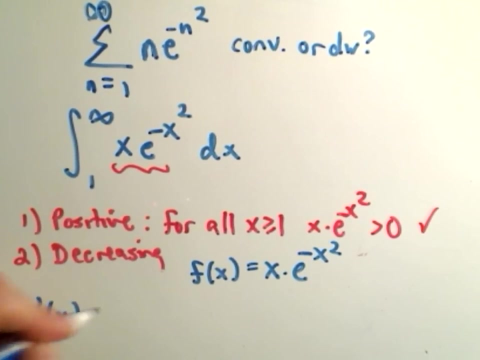 you know we have X, e to the negative x squared. you know, intuitively, maybe you can convince yourself it's decreasing. but the idea is to show something's decreasing again, you have to use the first derivative. so here's our function: we have to take the first derivative of this. we'll get f, prime of X, so the 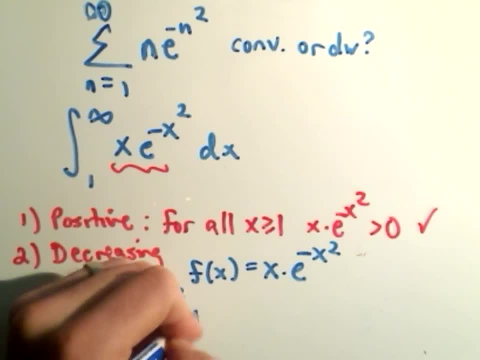 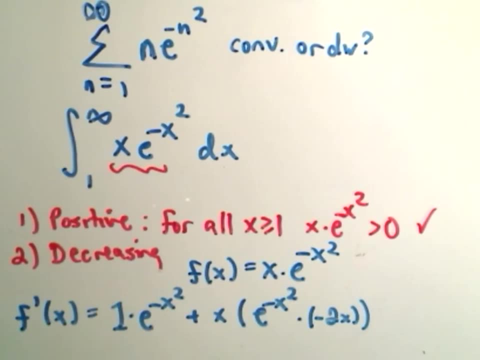 derivative of X is 1, we'll leave the e to the negative x squared alone, plus leave the X alone. we'll get e to the negative x squared times negative 2x, because we have to take the derivative of the exponent when we take the derivative of e. so I'm going to factor out the e to the negative x squared. 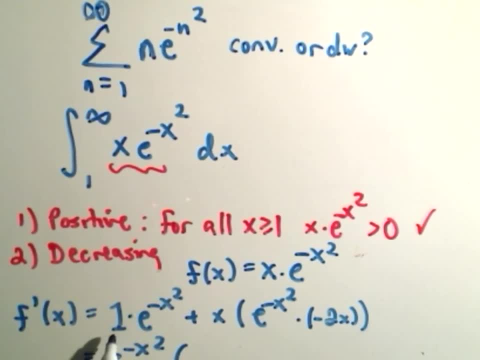 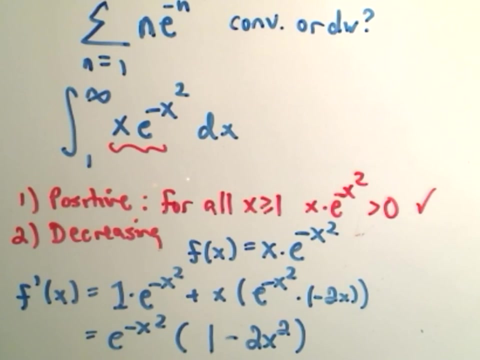 here and it looks like we would be left with a 1, and then, I think, over here we would be left with a minus 2x squared. okay, so that's the first derivative. whoops, sorry, got a little cut off there for a second. I got involved in my math, okay, so okay. 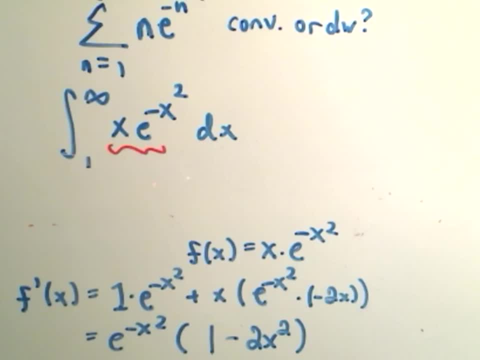 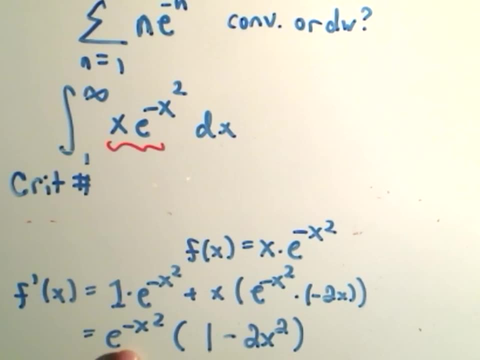 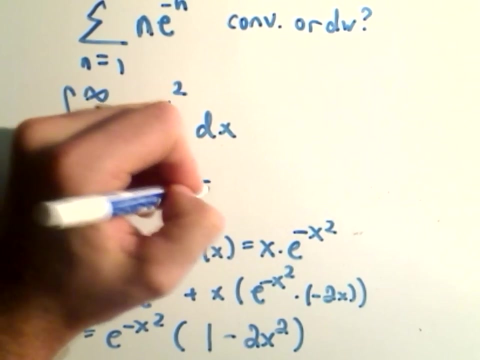 so what we have to do now is find the critical numbers of this. so the critical numbers where the negative xi elevates to the negative x squared is where the derivative of z equals zero, remember, or it's undefined. well, there's no place where it's undefined either. the negative x squared, again, is always positive. so 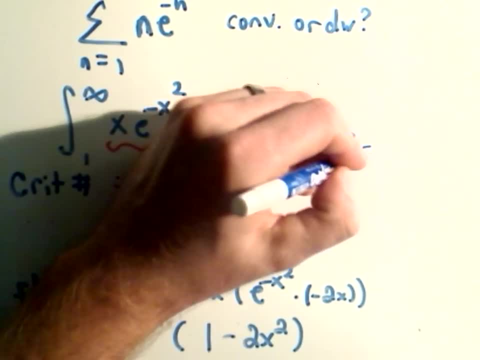 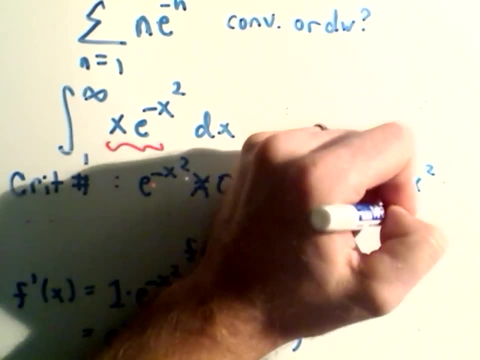 there's simply no solutions to that part. if we set the other part, 1 minus 2x squared, equal to 0, we can add 2, so we'll get 1 equals- excuse me why- the 2x squared divide and we'll get 1 half equals x squared. or if we take the sqrt minus 1, so 5x squared is 1.5, 1 minus 1 is 0. 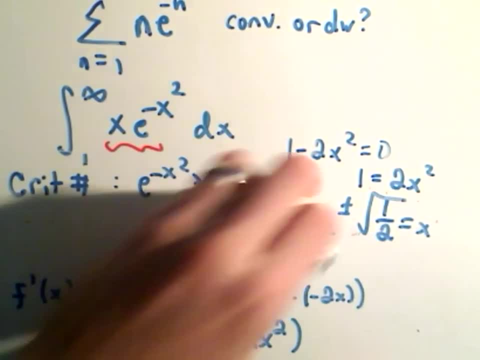 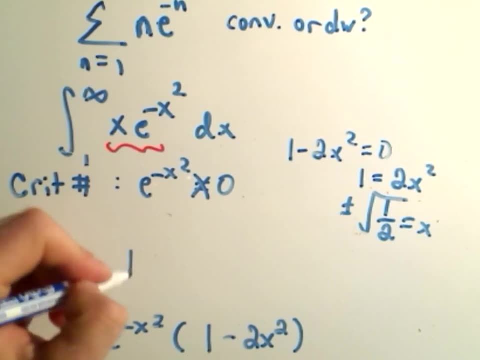 square root, we'll get positive, negative, one over root two. So those are going to be the critical numbers. here Again, I want to keep the derivative, but I'm going to keep it in factored form. Okay, so we're only going from one. 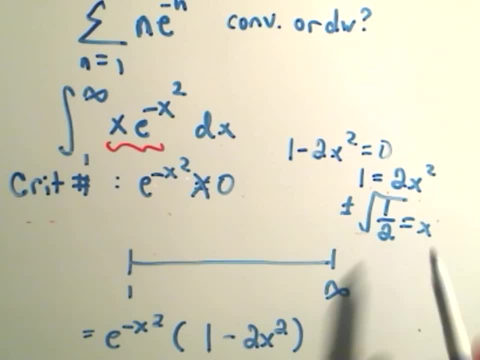 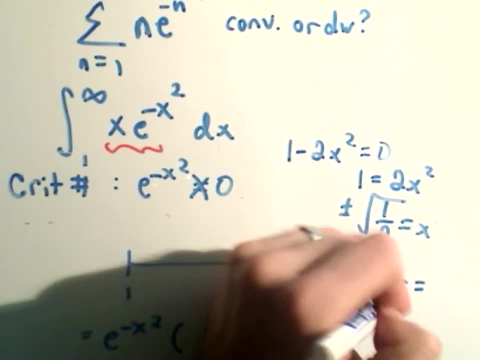 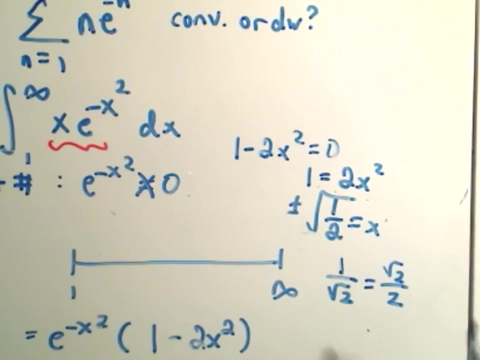 to infinity anyway. Well, this is going to be the number. we only need the positive part. so one over square root of two, or if you rationalize equivalently, we'll get square root of two over two, The square root of two. 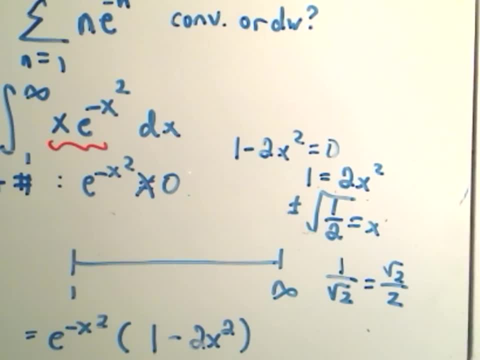 is certainly smaller than two, so this number is actually less than two. so really all we need to do is take any number greater than one and plug it into our derivative to justify that this is decreasing. So you may want to look over first derivative stuff. 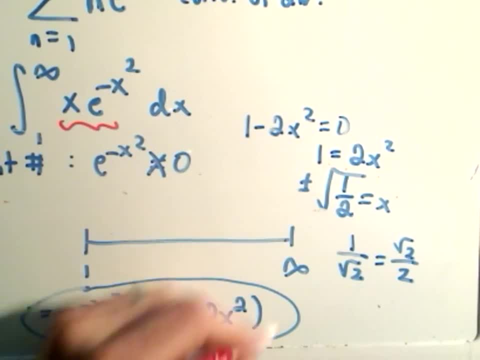 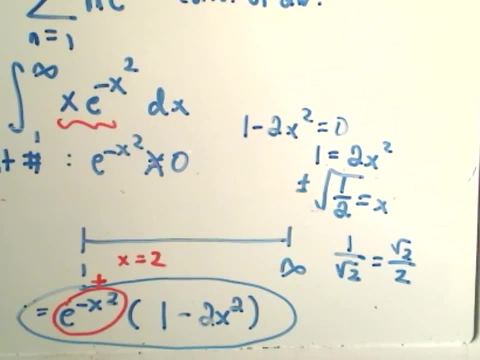 I've actually got some videos of that too, to find out where a function is increasing and decreasing. If you plug in, x equals two. again, notice e to the negative, x squared, that's always positive. On the part over here we'll get one minus what eight. 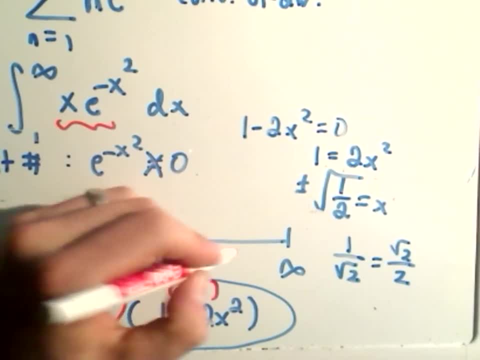 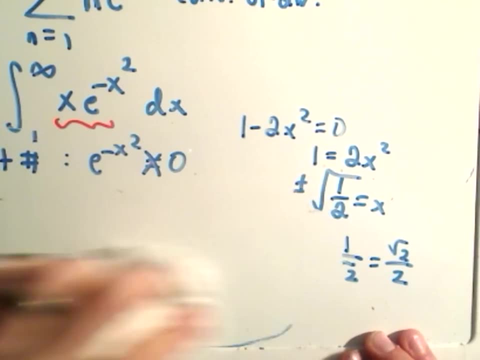 that's going to give us a negative number. so certainly it's negative over this interval, which means the function is decreasing. Okay, so the second condition is also satisfied. so we've now shown it's positive and decreasing, which means basically we're allowed. 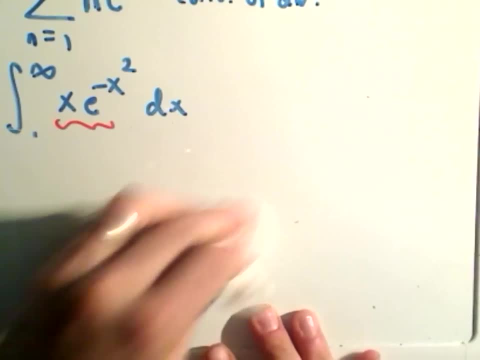 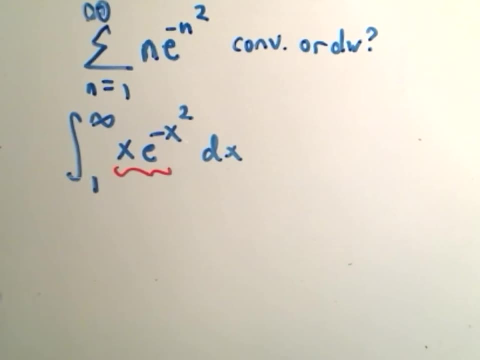 to do the integral test on it. So again, this is why I typically don't use the integral test, because it's pretty long. It's basically just a way to justify things all the way out. So I'm going to integrate the improper integral and then I'll just tag the limits back in there. 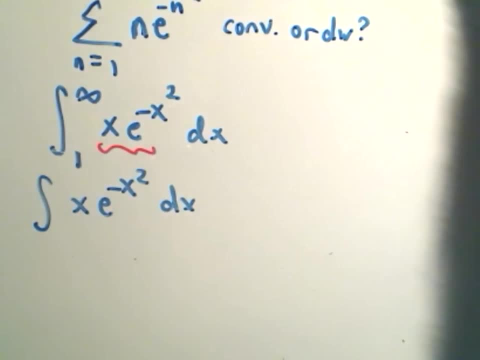 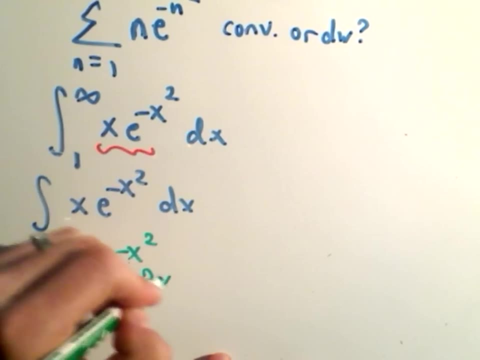 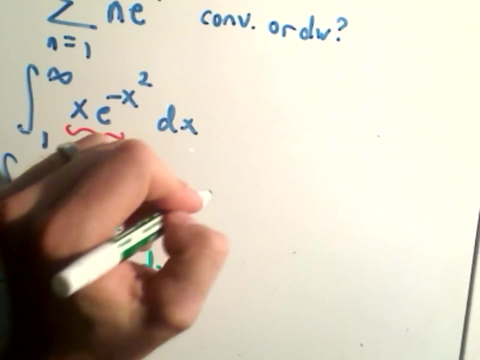 So I'm going to do a u substitution here. I would let u equal negative x squared. The derivative of that will be negative 2x dx. so divide by negative 1 half, you get x dx. So when we go to rewrite our integral with our substitution we'll get e to the u and again. 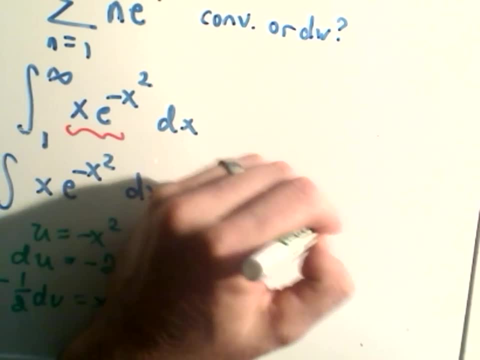 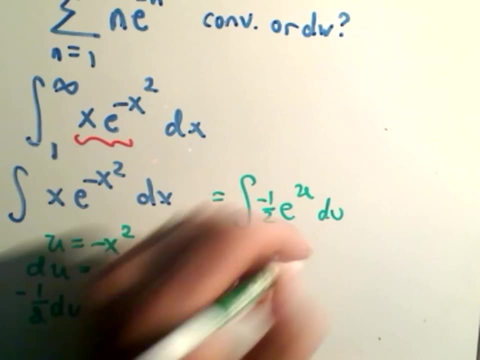 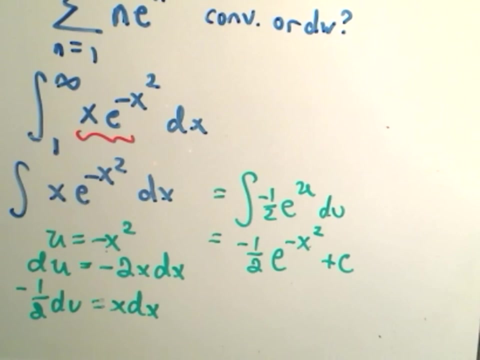 x. dx is being replaced by the negative 1 half du. When you integrate negative 1 half e to the u, you simply get negative 1 half e to the u, which again is negative x squared, And normally we would get plus c. but if I rewrite my integral, 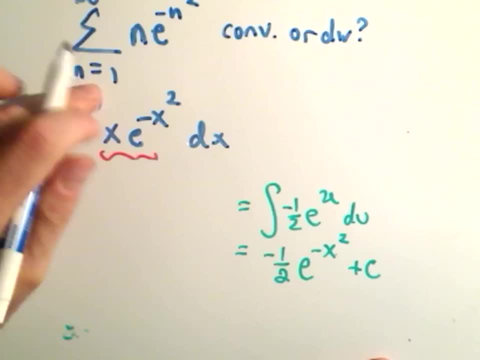 remember, when you have an integral from 1 to infinity, you'll replace the upper limit of integration with a t and then turn that into the limit as t goes up. Okay, Okay, Okay. So now I have this t squared and I'm going to calculate the limit as t goes to infinity. 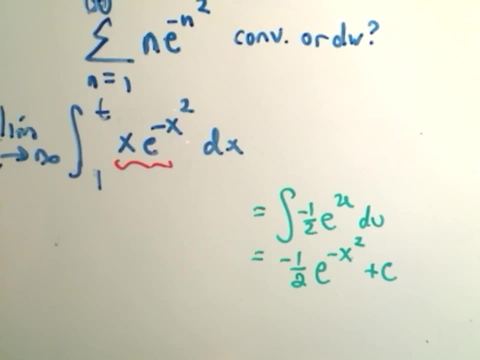 This is how we have to calculate improper integrals. So it says: really I'm going to calculate the limit as t goes to infinity of this thing, negative 1, half e to the negative x, squared from 1 to infinity. So these are long and hard. 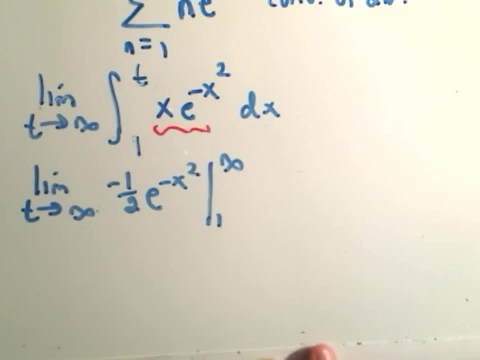 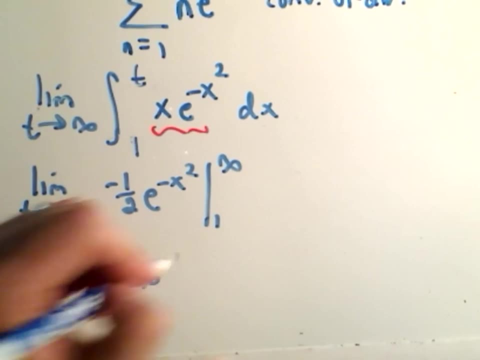 I mean it ties a bunch of things together for sure. That's why, again, I tried to avoid it. So this is going to be negative 1, half the limit. as t goes to infinity, We'll get e to the whoops I plugged in. 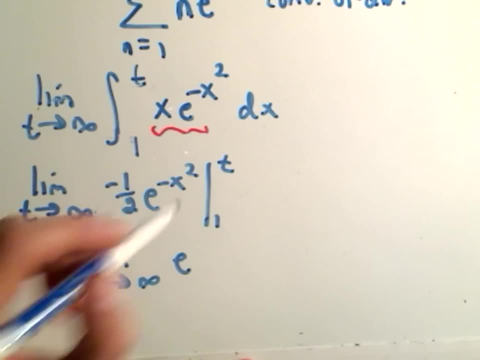 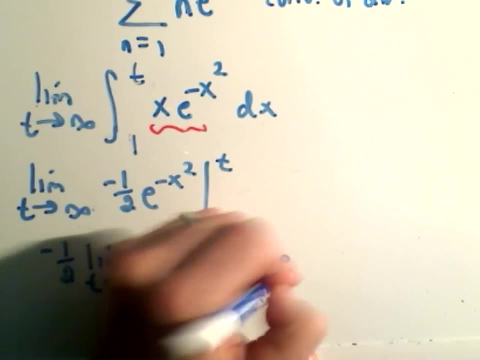 I put an infinity in here and I need a t. So pull the negative 1 half out. We'll get e to the negative t squared minus. when I plug in 1, I'll get e to the minus 1.. So again, I'm just pulling the negative 1 half out front. 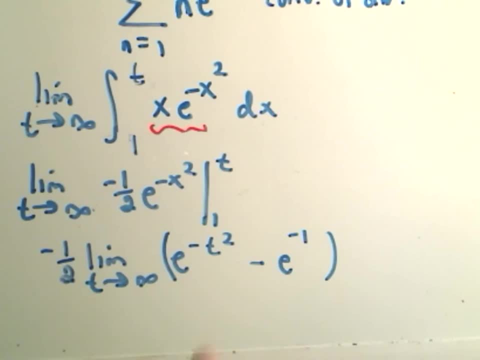 plugging the t in plugging the 1 in. Well, again, if this integral is convergent, that means it equals some finite number. then the series also converges: e to the negative first, e to the first is just a constant, so I'm really not worried about that part. 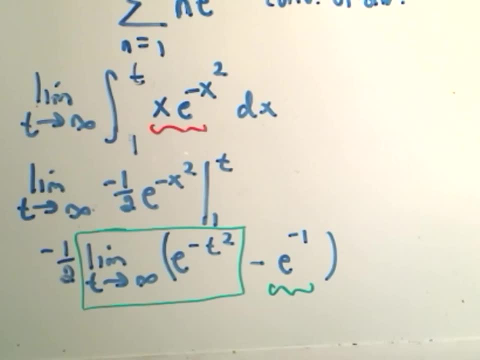 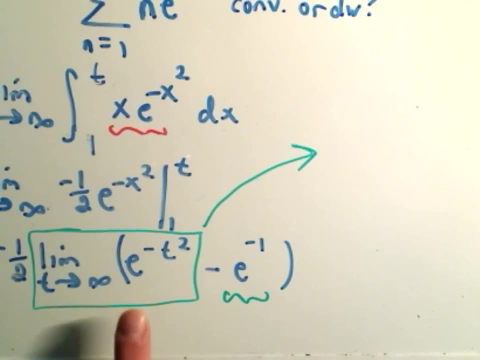 I'm just really kind of interested now in what happens to the limit as t goes to infinity, of e to the negative t squared, Because if that's a number, it'll all turn out to be a number, which means it's convergent. 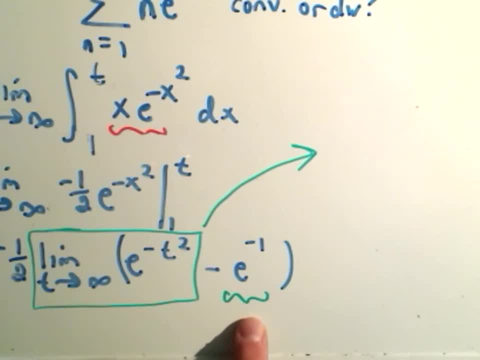 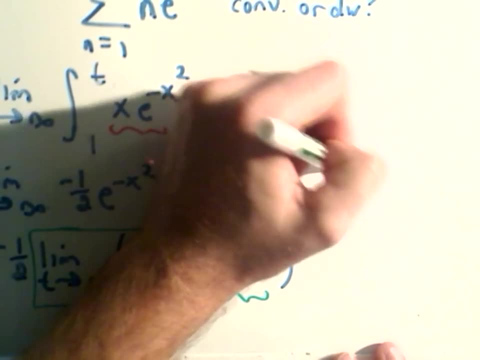 If this goes to infinity or negative infinity, well, who cares? If you're subtracting away a finite number, it'll be infinite, and that means it diverges. Well, to calculate this limit, this is just the limit, as t goes to infinity. 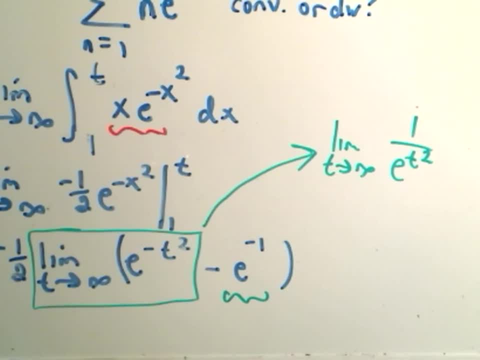 of 1 over e to the positive t squared, And you could even calculate this directly. I think this is sometimes more clear to people, So I just move it to the bottom. by making the exponent negative. As t goes to infinity, we're going to get e to a large number. 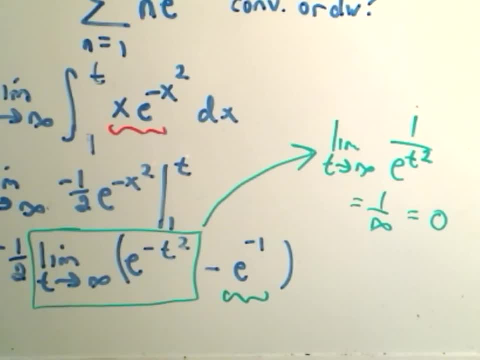 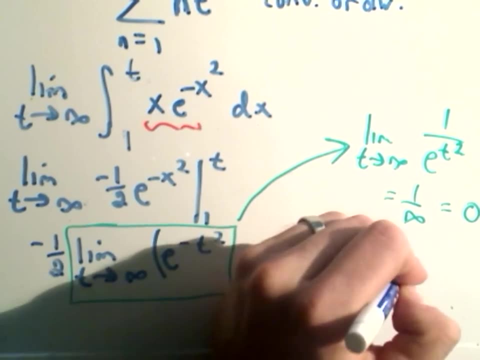 Well, 1 over a big number is 0. So it says this improper integral. we've still got the negative 1 half out front, so we'll actually get positive 1 half e to the minus 1, or 1 over 2e. 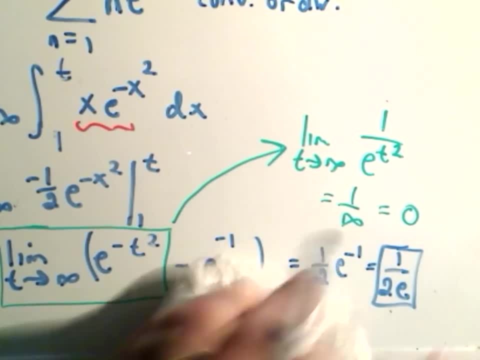 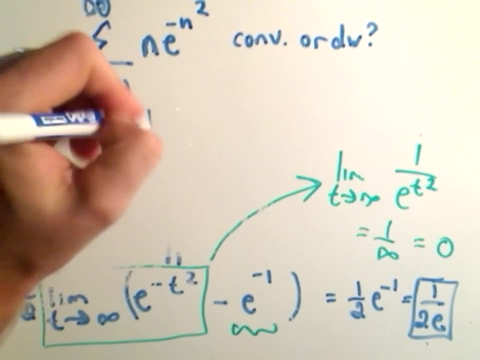 So it says the integral converges, And since we know now that the the integral converges by everything that we've shown, we can justify that this series also converges. Don't make the mistake, though, and say that this series converges. 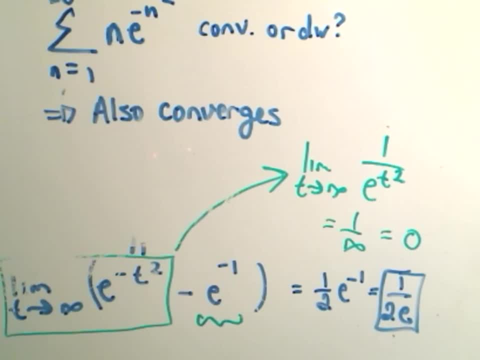 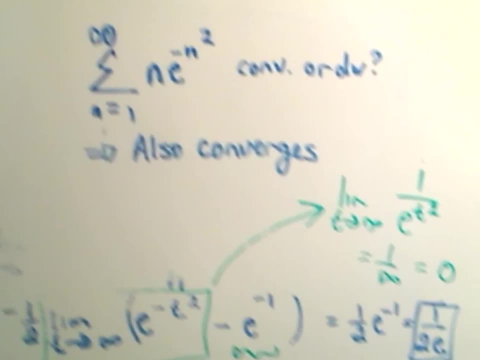 to 1 over 2e the value that we found, because that's not correct at all. Okay, that's definitely not true. But we can say: if the improper integral's convergent, so also is the original series.